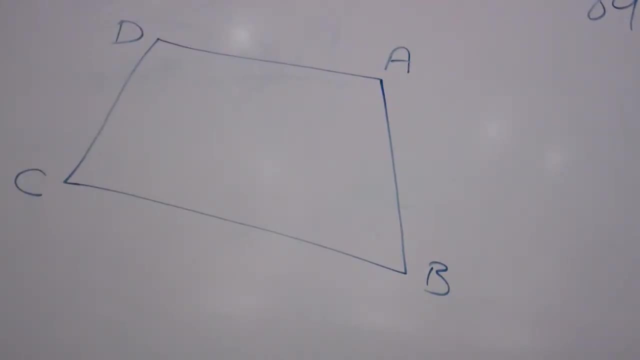 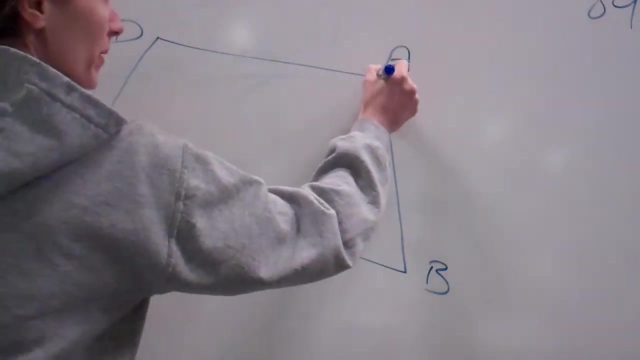 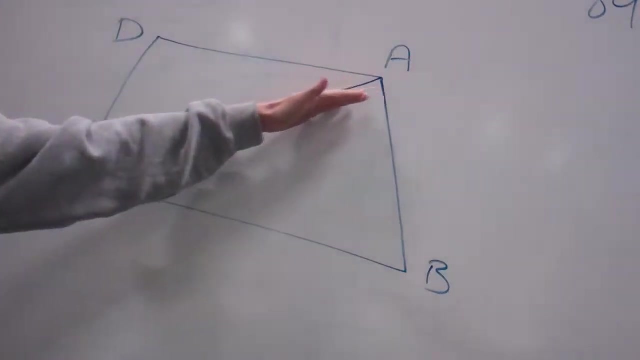 Now a diagonal. what you're going to do is draw a diagonal between two non-adjacent angles, And a non-adjacent angle is basically like opposites- It's not on the same side- Okay. So non-adjacent would be the opposite of A, which would be C. You see what I'm saying? So we're going to draw a diagonal right here, non-adjacent vertices, both of them, Okay. 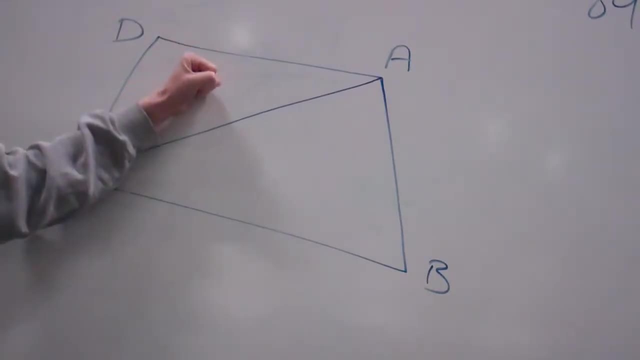 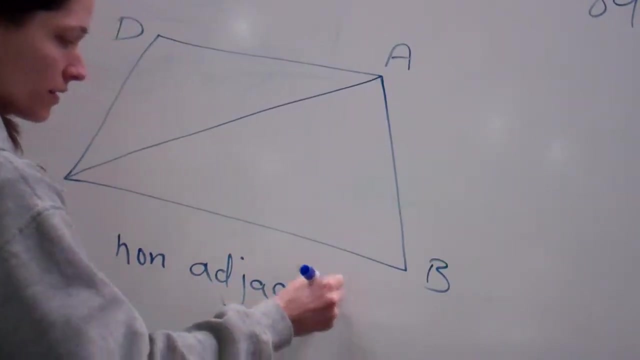 Now, what do we know about triangles? Non-adjacent, Just like that. Okay, All right. So if I were to put a diagonal down here, does that help me? Yes, it does, And I want you to see why. 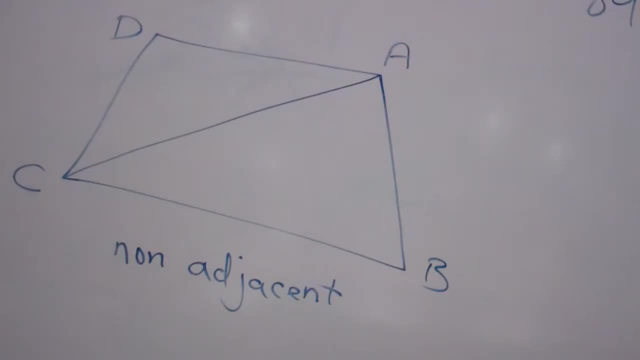 This is a triangle and this is a triangle. And what do we know about triangles? They have three sides. They do have three sides. They do have three sides. Perfect, This one is 180 degrees and this one is 180 degrees. Everybody see that and understand that. Okay, 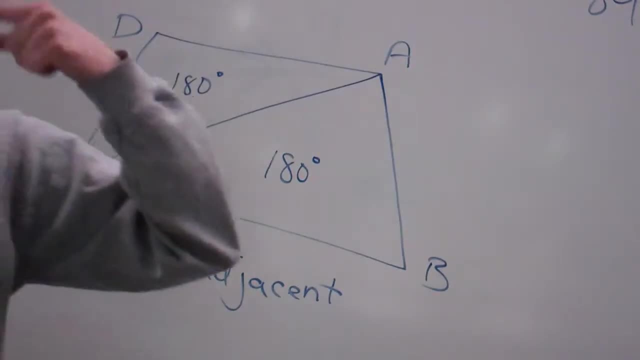 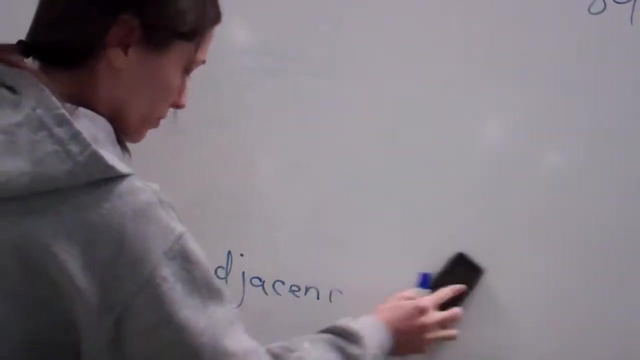 So us just knowing information about triangles is going to help us in this, Okay. So now let's look at a different shape. That's just kind of the beginning I just wanted to show you. Okay. The next thing I want you to draw is a hexagon, Okay, And a hexagon has how many sides? 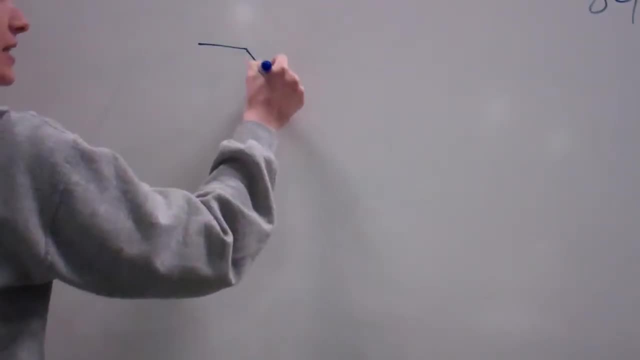 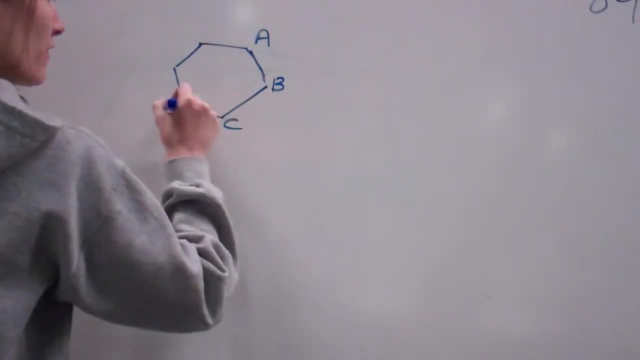 Six, Six, Hex. It's kind of like six, One, two, three, four, five, six. Now they said that this is a regular hexagon. What does that indicate? They're all equal. Very good, Regular means that they're all equal. Okay. Now, because I'm human, I have imperfections. Therefore, this does not look like a regular hexagon. It looks kind of messed up, Okay. 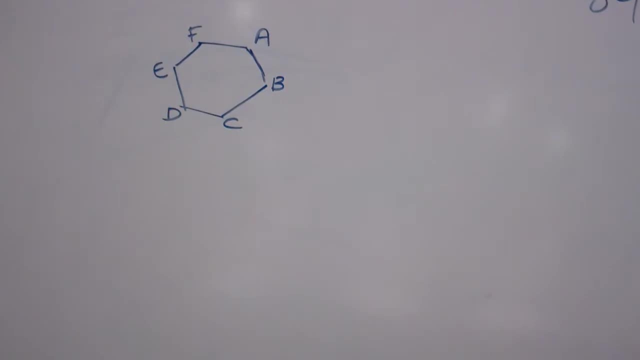 So everybody draw a line. Everybody draw one of those A through F on there. Okay, Now what you're going to do is you're just going to pick one vertices. Okay, Does anybody remember what a vertices is A line? 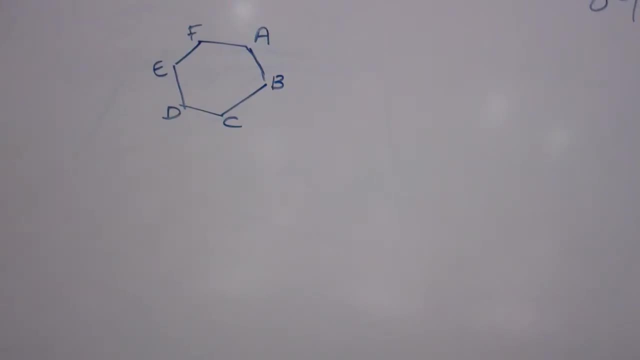 Where they meet, Basically the points. Okay, So you're going to pick one of them. I'm just going to pick A because I start with A. Okay, So this is the one I'm going to work with, And what you're going to do is you're going to draw from A to each non-adjacent Okay, So watch what I do. 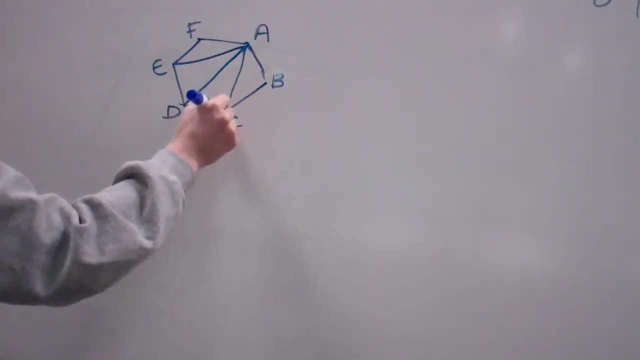 I'm going to go boom, Boom, Boom And boom. This is going to be very helpful in what we discover in just a minute. So how much degrees does this entire thing make up? Let's figure it out. This triangle is. 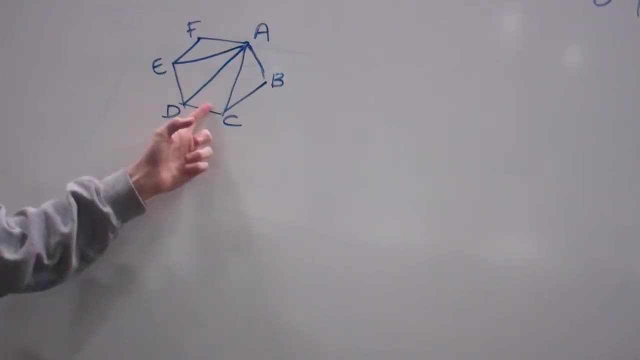 180. 180. 180. 180,, 180, 180.. 104 of them equals 720.. Okay, So each of these- and I'm only going to write the first one- is 180 degrees. Now I'm going to take away my lines for just a minute and I want you all to see what happens. 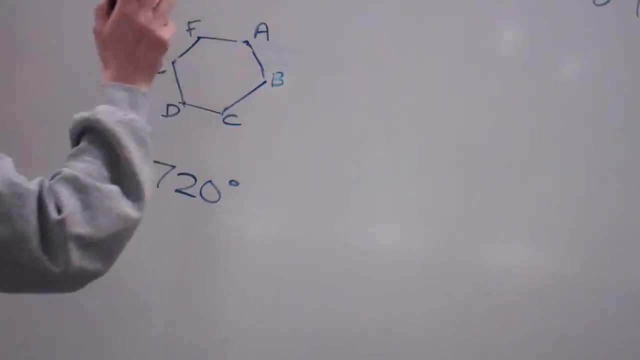 So, because we know that each of these lines are regular, it also means that each of the angles are regular, which means what Regular? They're all going to equal the same thing. So this angle is just the same as this angle. 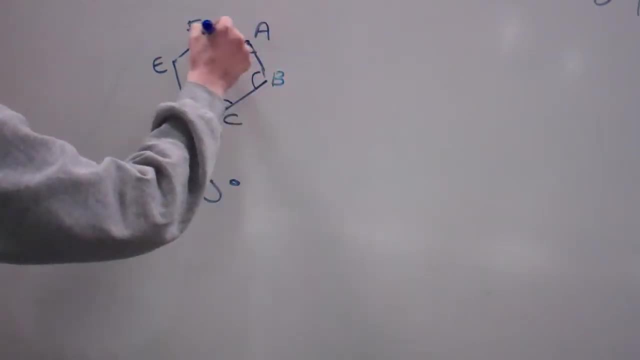 It's just the same as this angle. Okay, Every angle is the same because it's a regular hexagon. Okay, How do I figure out what each angle is if I know the total is 720?? Very good, Lane. So because we have six angles and we know that the total inside- because we did diagonals, we broke it up- equals 720.. 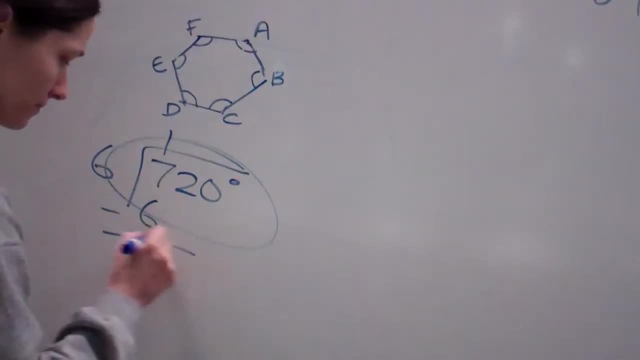 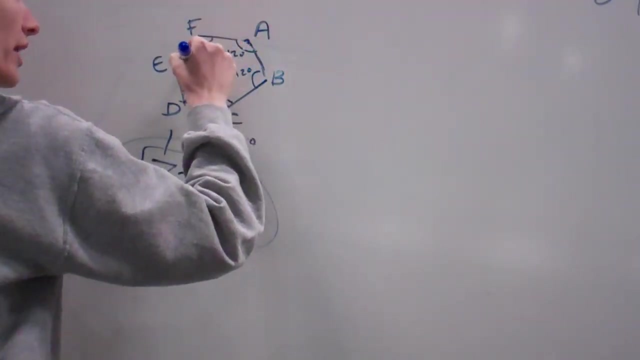 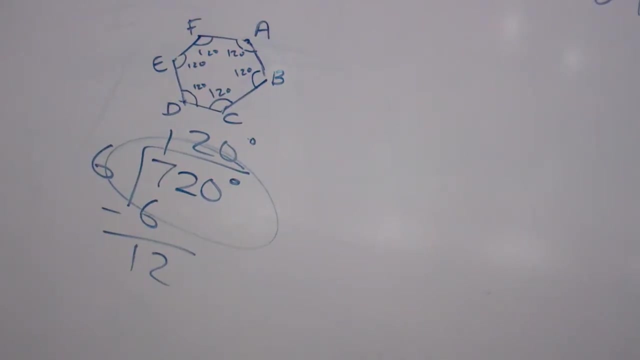 So when I do that, I end up getting 120.. So each of these is going to equal 120.. Okay, Everybody see how we did that, How we discovered it. Yes, Okay, That is learning how to do interior angles. 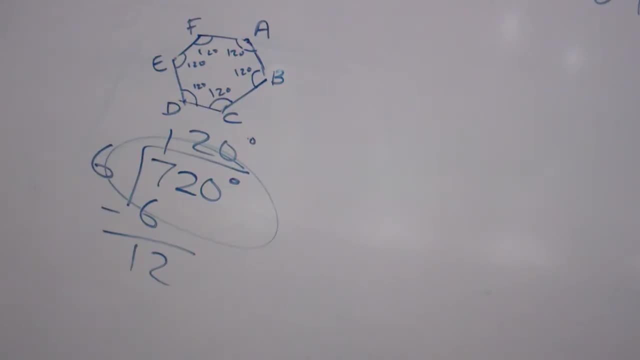 Okay, And I'm going to go on and do a few more, and then we're going to learn about exterior angles, Okay, So I'm going to leave this one up here for just a minute, Okay, Because I want to use it again. 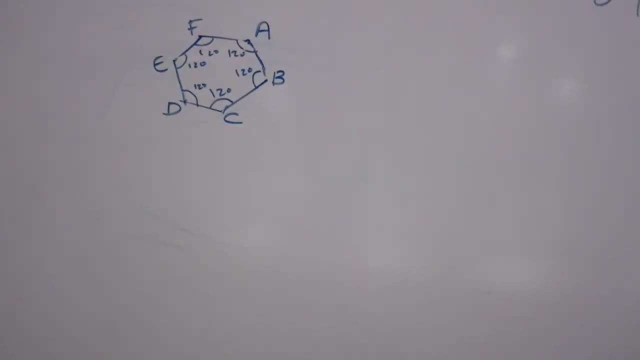 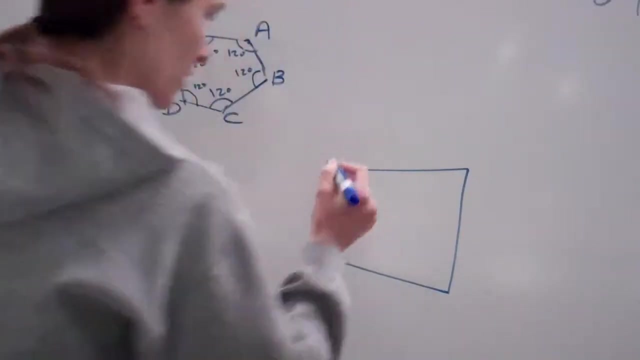 Okay, But let's go on and do another problem, All right. So, for example, if I, this is kind of like the one we drew in the very beginning, Okay, Actually, it goes out just a tad bit more, There we go. 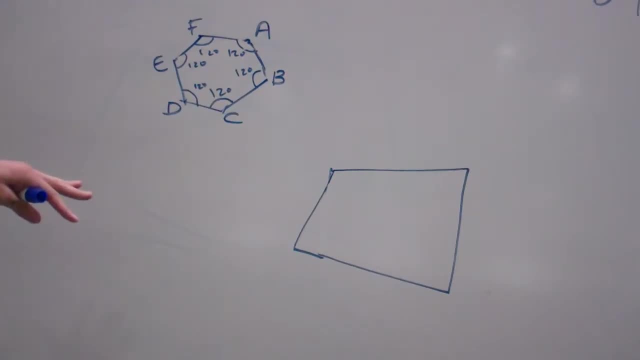 Okay, And here's what it says: Draw a quadrilateral and one of its diagonals. So I'm going to draw a diagonal, Okay, So I drew a quadrilateral, four-sided shape, and then I drew one of its diagonals. 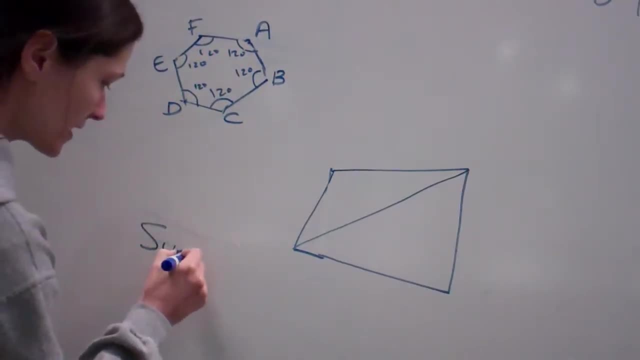 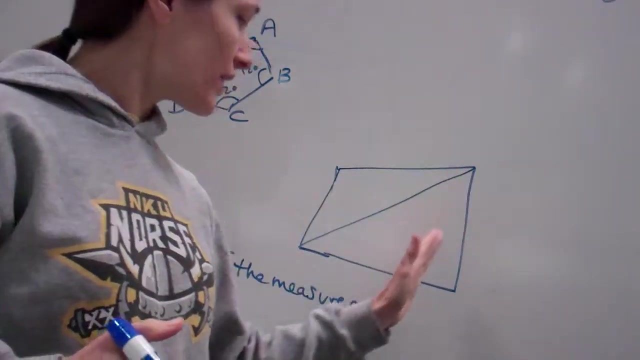 Then it says: what is the sum? what is the sum of the measures, What is the sum of the measures of the interior angles of this quadrilateral? So they're saying: what do all of these equal together? What do you mean? 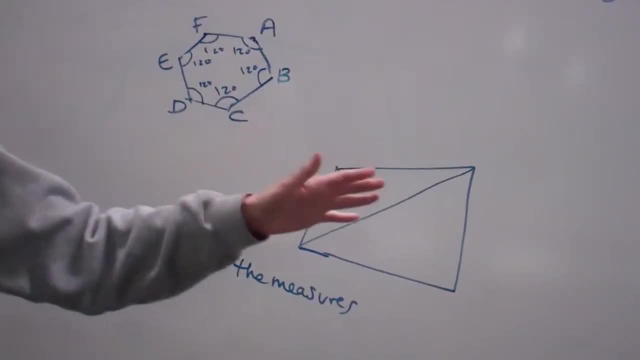 Like both triangles, All the triangles, Both. Well, that's eventually Okay. So what you're going to do is we're going to try to figure out. this triangle is how much? 180.. 180. And this triangle is what. 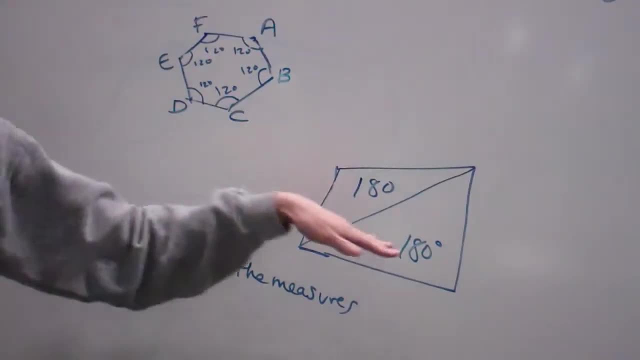 180.. Okay, So what is the sum of the total inside 360.. Okay, So that was pretty easy. Okay, But that's some of the questions you're going to hear. All right, They're going to ask. 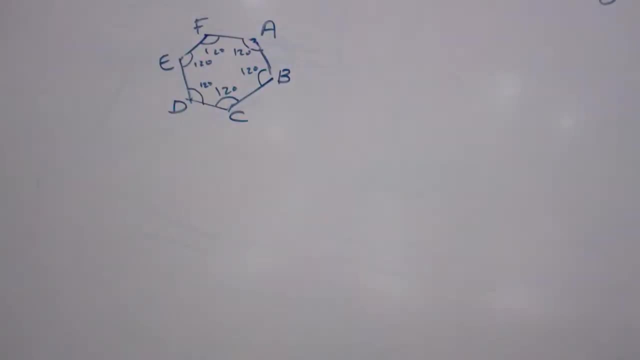 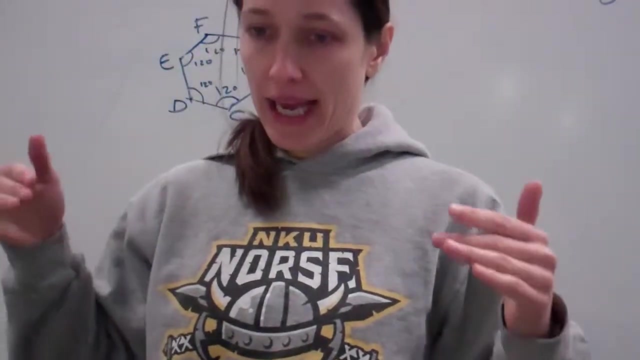 All right Now. hopefully you remember that sum meant to add and get your answer. All right Now let's look at exterior angles. Okay, Okay. So If I decide to go for a walk and I start in this place and I were to walk around lane, 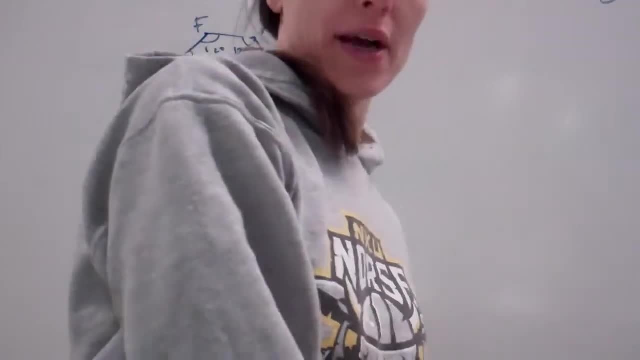 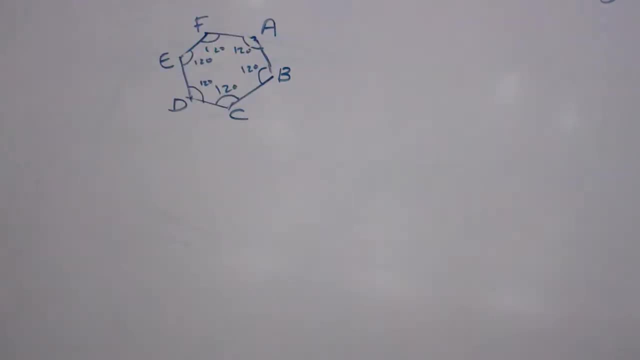 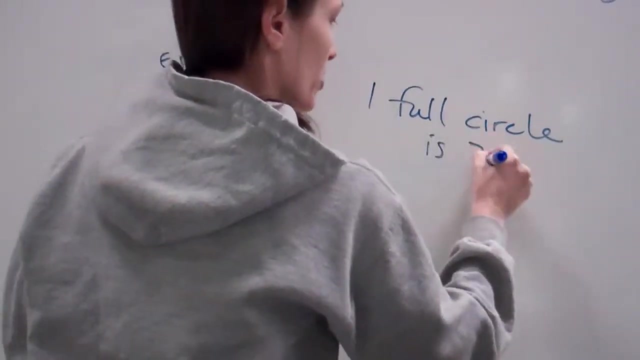 around that outside and then come right back to the spot I am. what does one full circle make in a degree 360.. Very good for you to know. Okay, So one full circle is 360 degrees. If you don't already know that, write that down. 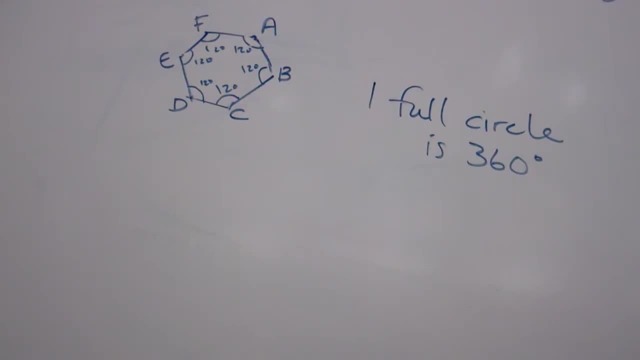 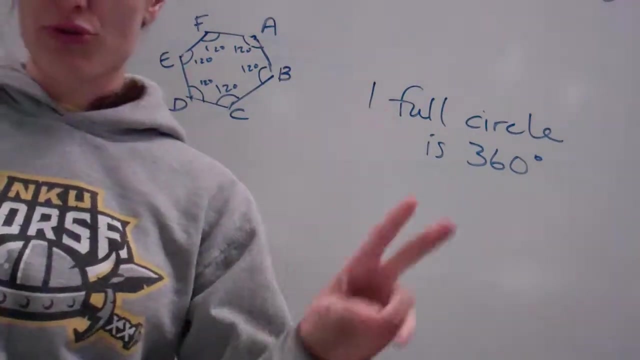 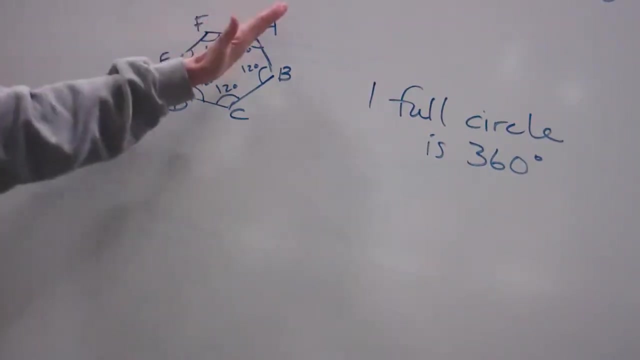 It's very important. Now there are two ways that you can figure out the answer to this. what I'm fixing to say: Okay, And what I draw actually looks really cool, Okay. So what you're going to do, let's say I'm at A and I'm going towards B. 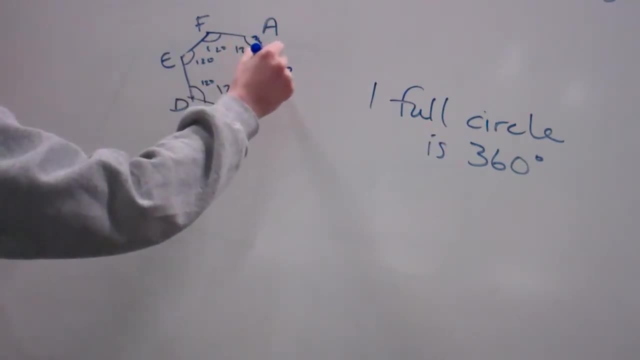 Okay, So here I am, Dun dun, dun, dun, dun dun, Walk, walk, walk, walk, walk. Okay. Okay, If I went straight, that's where it would go. Okay, So I would just keep going, but instead it turned. 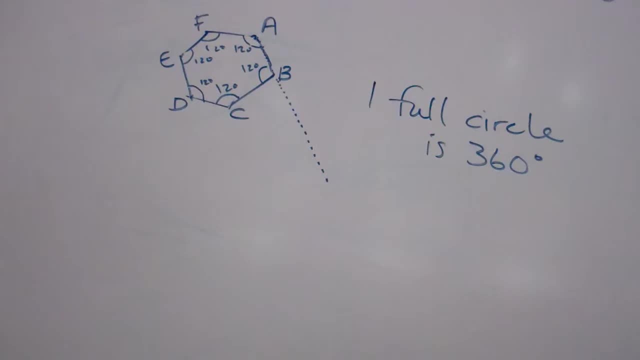 Okay, I'm going to turn at B and start walking towards C. So I start walking, start walking, start walking. Okay, If I did not turn and I kept going, that's what it would look like. Okay, But I turned. 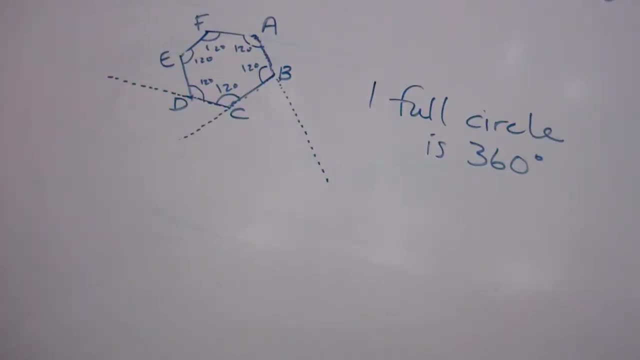 So now I'm going to go towards D- Okay, And then towards E, And then towards F, Then towards A- Okay. What you get is this cool looking like star, like almost like something you'd see on some kind of ninja show or something. 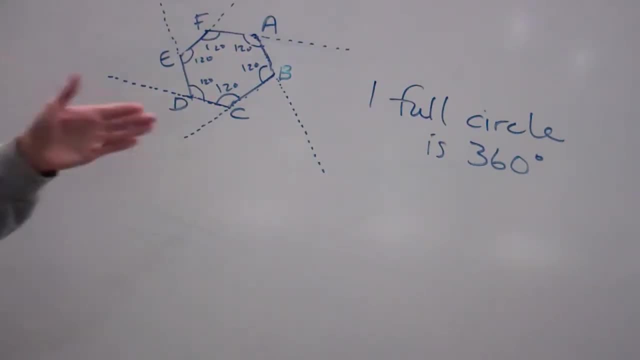 It's like spinning. Okay, It looks kind of cool. But what I want you to see is what did I actually make just by going straight? I made exterior angles. Does everybody see That's an angle, This is an angle. So basically I'm saying let's go from A to B, and then how much did I turn? 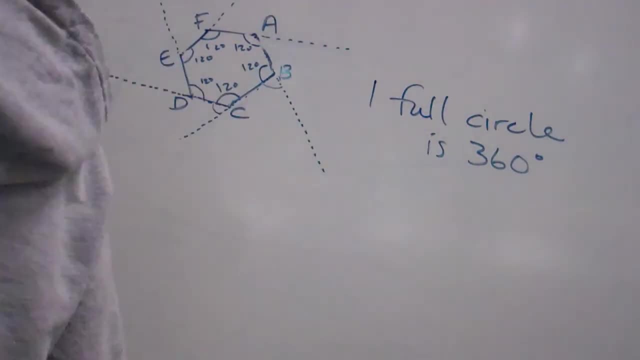 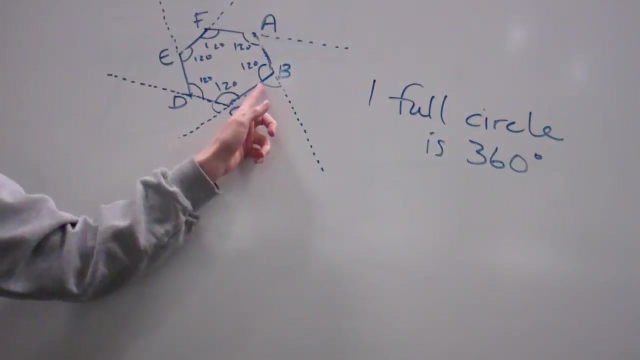 Instead of keeping going straight. how much did I turn in my angle right here? Okay, So if I'm walking from A to B and instead of keep going straight, I decided to turn And I want to know how much degrees did I turn? is basically what I'm doing. 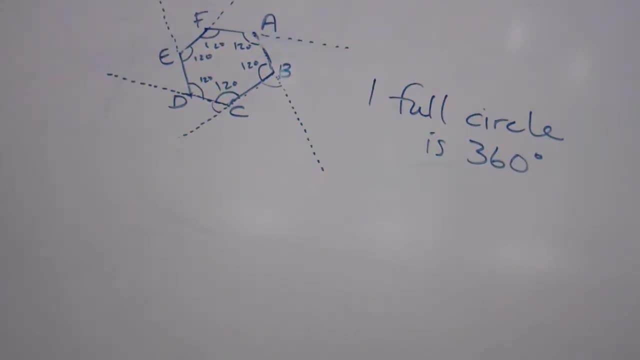 So there are two ways to discover this. Okay, I know that one full circle equals 360 degrees, And if I have 1,, 2,, 3,, 4,, 5, 6 exterior angles, how much will each exterior angle be? 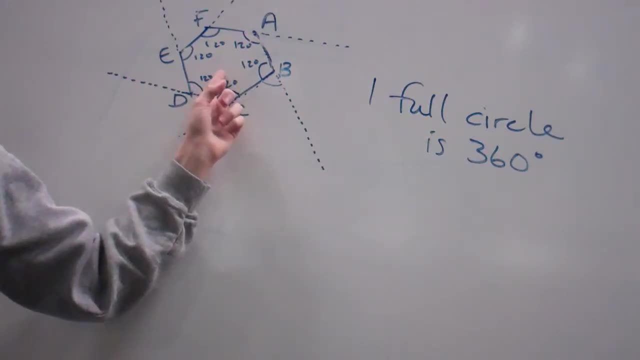 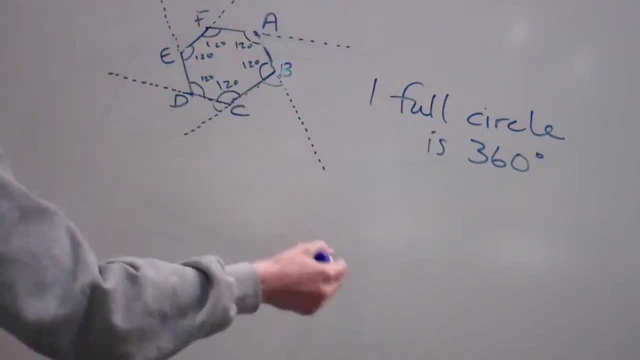 Now that was when it was 720 on the inside, 60. 60.. Because I have 360 total to go from A to B. I know it's going to be 360. Okay, But how many times did I turn? 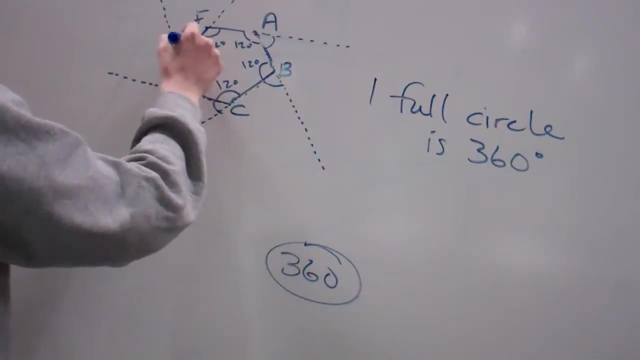 1, 2,, 3, 4.. 1,, 2, 3, 4,, 5, 6.. I turned six times, So instead of walking continually and not turning at B- okay, I would have kept going straight. 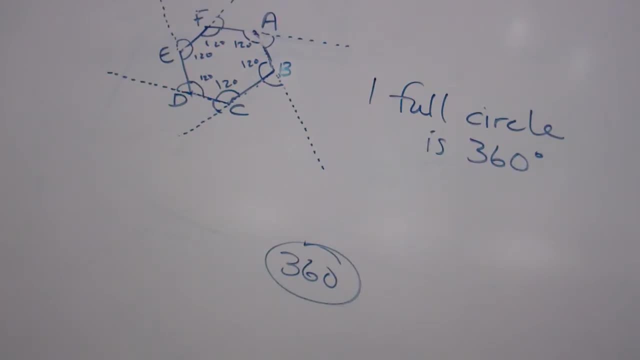 But this time I'm going to keep walking, and instead of keep walking straight, I'm going to turn. How much did I turn to then begin walking from B to C, 160 degrees. Okay, Each time I turned, I turned my body 60 degrees.